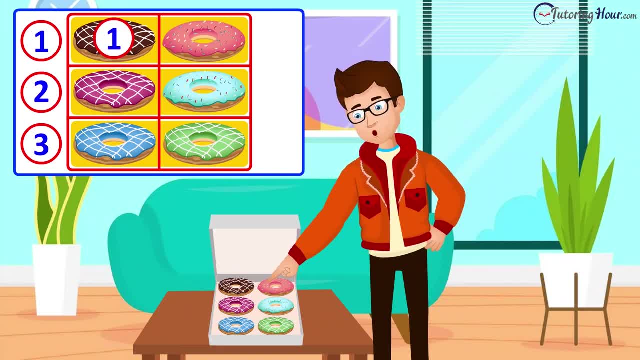 How many donuts are in each row? One, two. There are two donuts in each row. To find how many donuts there are, we can either count the donuts one, two, three, four, five and six, or add two plus two plus two. 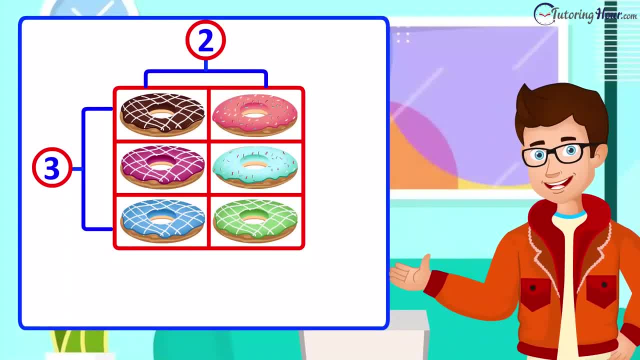 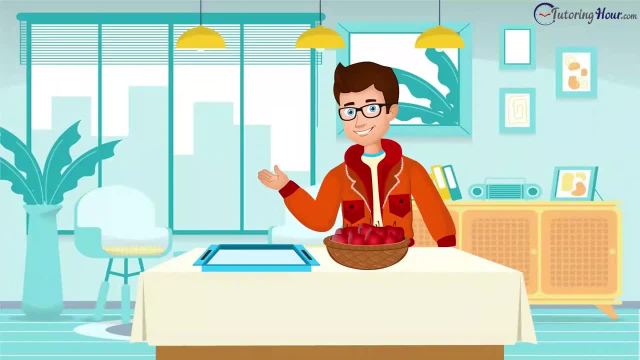 We can also view the array as three groups of two donuts and form the multiplication equation as three times three. The answer is six donuts. Let's move on to creating an array of apples for the problem three times four. Here's my basket of apples. 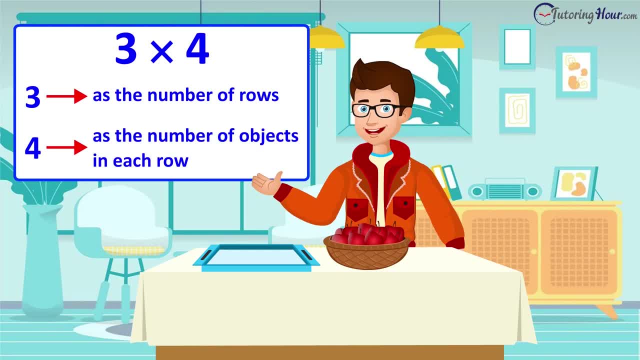 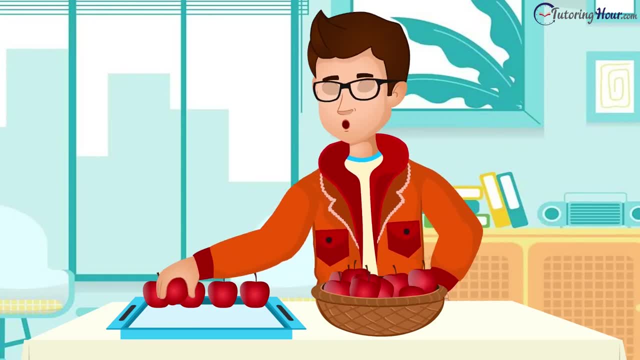 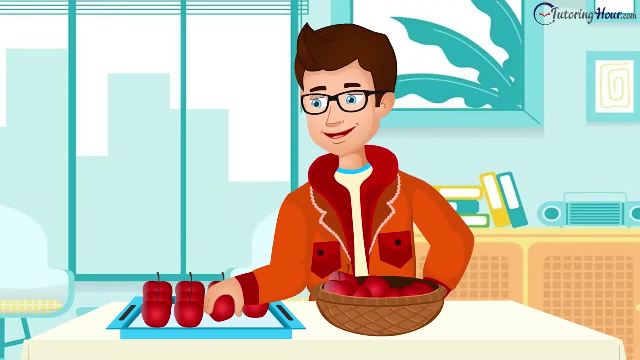 We take three as the number of rows and four as the number of objects in each row. I'll put one, two, three and four apples in the first row, One, two, three and four apples in the second, And one, two, three and four apples in the third. 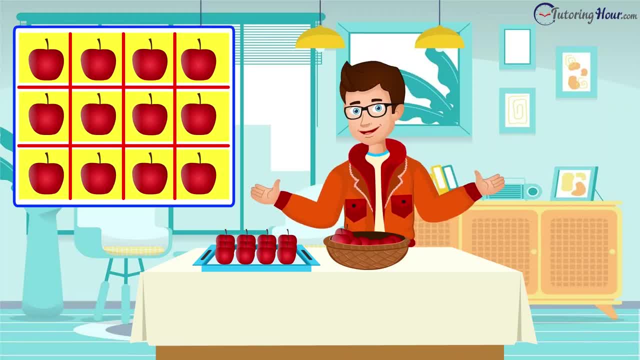 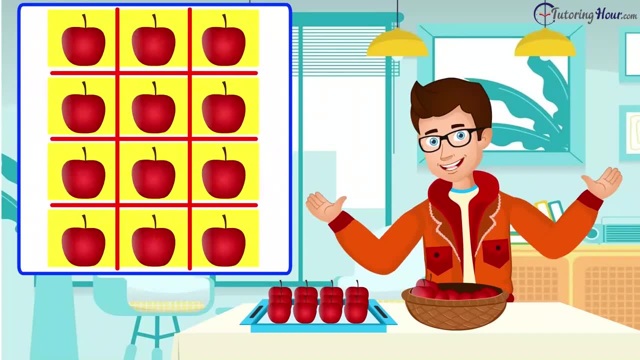 Here's our array of three rows with four apples in each. Let's put this in a multiplication sentence: Three times four is equal to twelve. Let's try flipping our array Now. we'll have four as the number of rows and three as the number of apples in each row. 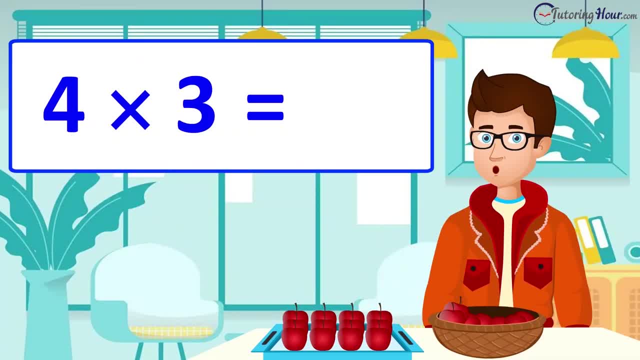 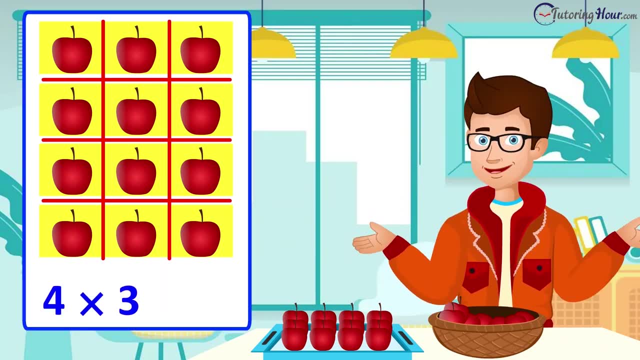 The equation would be: four times three is equal to twelve. The array would look like this: The number of apples, however, would remain the same, as four times three is also equal to twelve. Changing the order of factors in the equation wouldn't change the product. 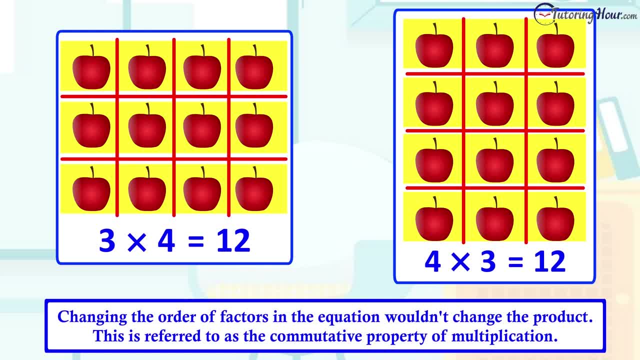 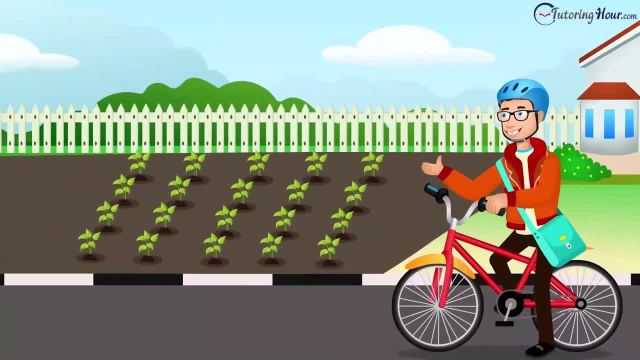 This is referred to as the commutative property of multiplication. Let's explore and look around for some more real-life arrays. Did you see the saplings arranged neatly? Can you tell how many saplings there are? Let me pull out my book and build the multiplication equation first, 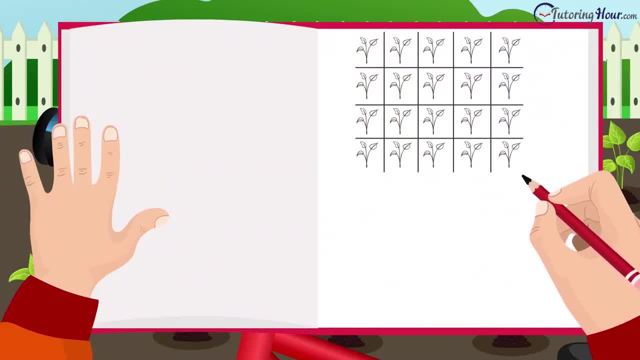 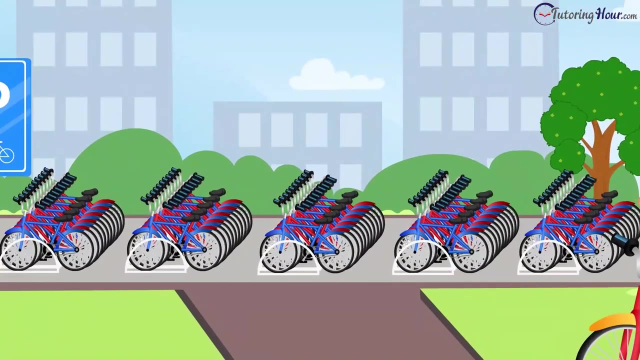 We have four rows with five saplings in each, so our multiplication sentence will be four times five, And what is the answer? Twenty. There are twenty saplings here. That was pretty quick. Let me park my bike. Do you see an array here? 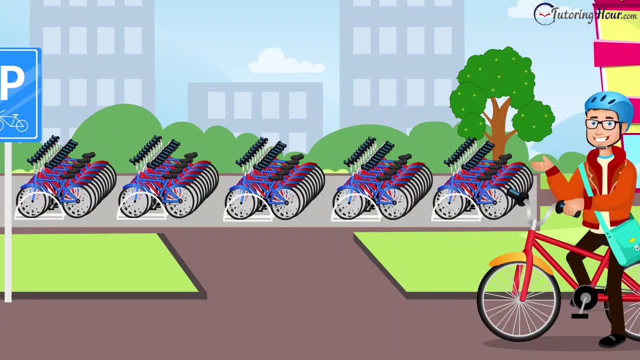 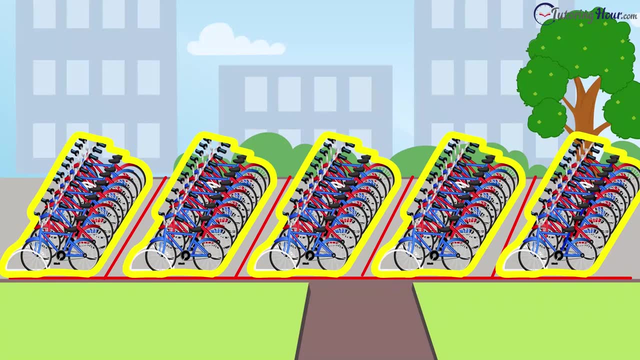 Can you tell how many bikes there are in all? Counting them one by one would be a tedious process, so what we can do instead is multiply. First, let's find out how many rows of bikes there are. We have five rows. How many bikes in each row?